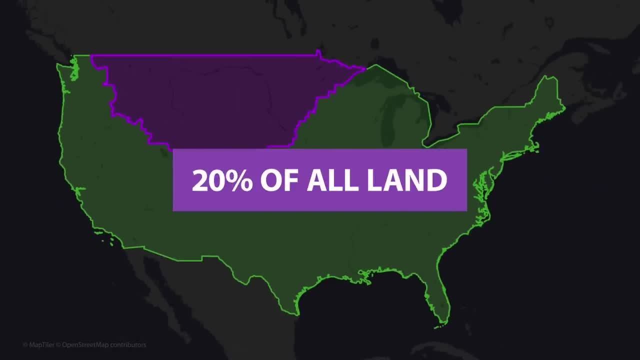 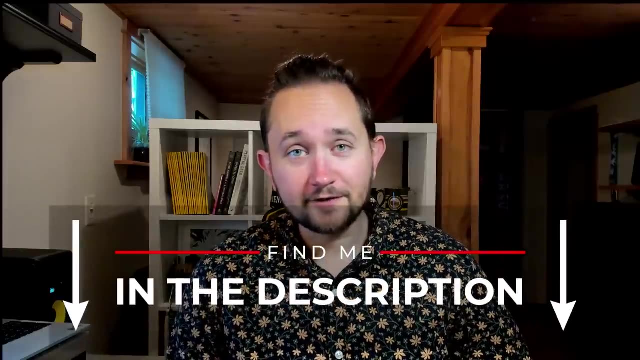 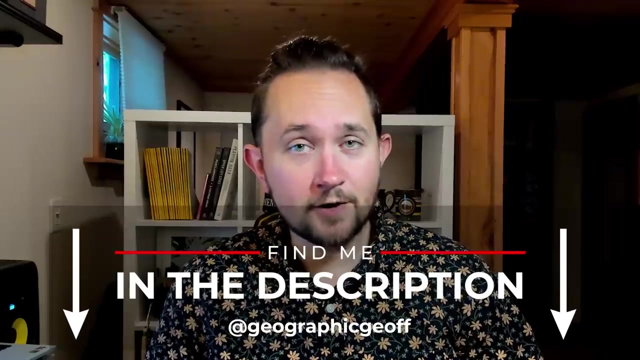 despite consisting of nearly 20% of the contiguous United States. Here's why, Hello and welcome to Geography by Jeff. Today we're off to explore another weird population distribution pattern in the United States. If you didn't know the region we're talking about. today largely consists of the Great Plains on one side and the Rocky Mountains on the other. This might make it seem inhospitable, but if we look even farther north into Canada, we see two major Canadian cities in Edmonton and Calgary. So why are there no major US cities? 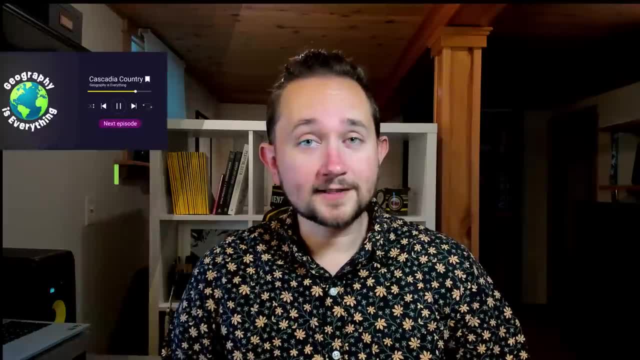 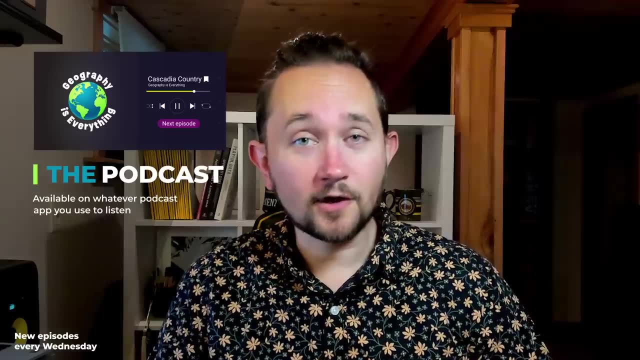 here We're about to find out, But before we explore why the US doesn't have a major population center in this region, be sure to check out my podcast: Geography is Everything. This week we're going to explore the incredible geography. 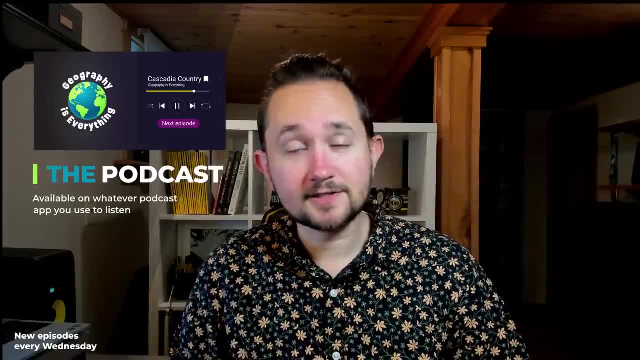 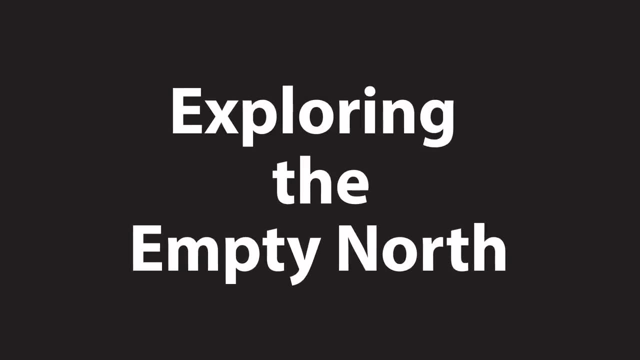 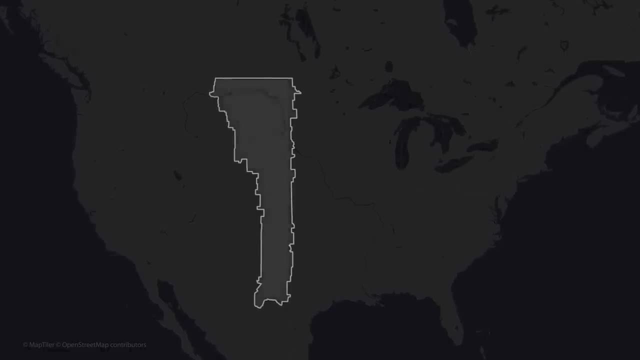 of T. You can listen to that episode right here on YouTube, Substack or whatever app you use to listen to podcasts. Those of you who watch my channel regularly are probably familiar with a video I created a few months ago where I looked at what I called America's Empty Belt And while that region still 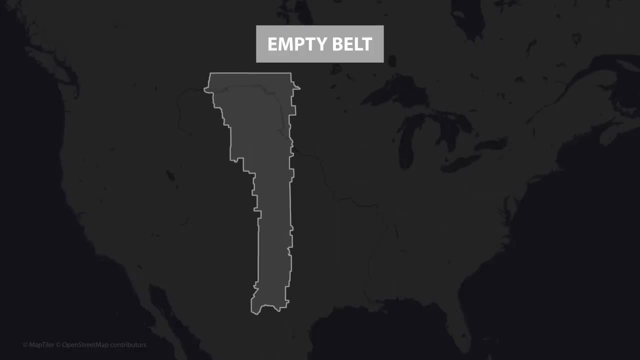 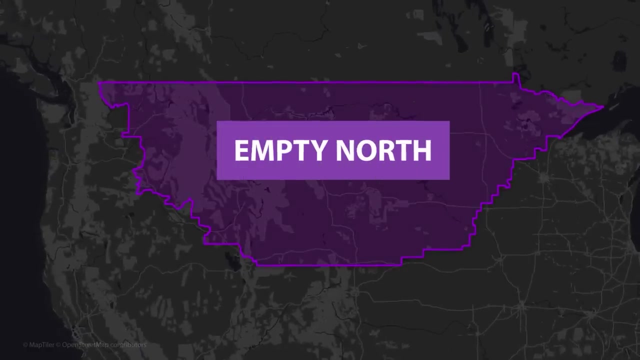 leads in terms of having the fewest people in the largest area in the contiguous United States. it led me to start looking at the northern region of the country as well, an area that I've termed the Empty Belt. The Empty North I've cobbled together consists of the full states of Montana. 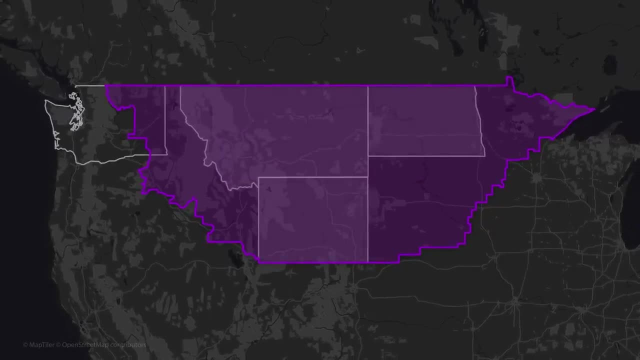 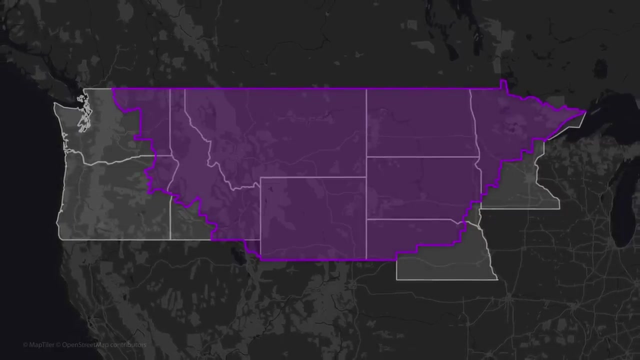 Wyoming and North Dakota, as well as portions of the states of Washington, Oregon, Idaho, Nebraska, South Dakota and Minnesota. All told, the Empty North of the United States takes up a gargantuan area of about 553,000 square miles. 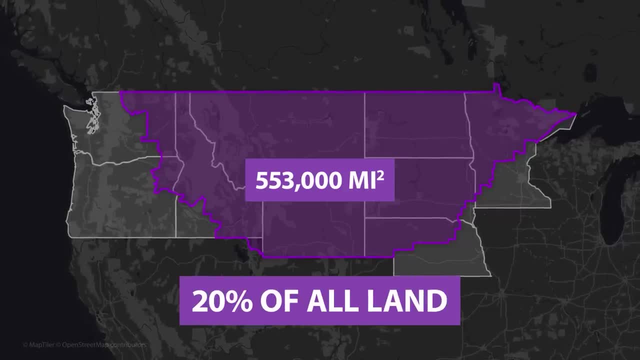 which would equate to nearly 20% of all land within the contiguous United States. Now, despite being such a large area, consisting of large parts of so many states, this entire area is a large area of about 553,000 square miles. The Empty North I've cobbled together consists of the full states of Montana. 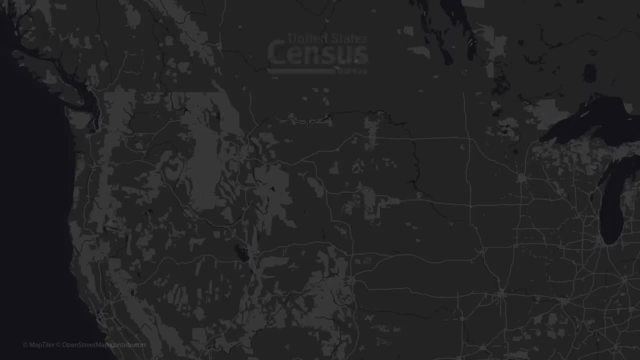 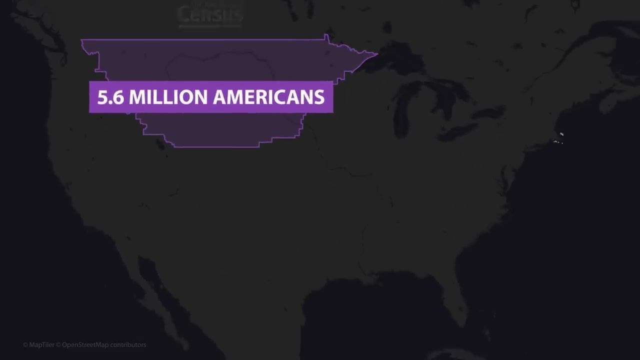 region has relatively very few people living in it. According to the latest US census, this region is home to approximately 5.6 million Americans. To put this in perspective, the state of Massachusetts, which is about 7,800 square miles, or about 1% of the size of the 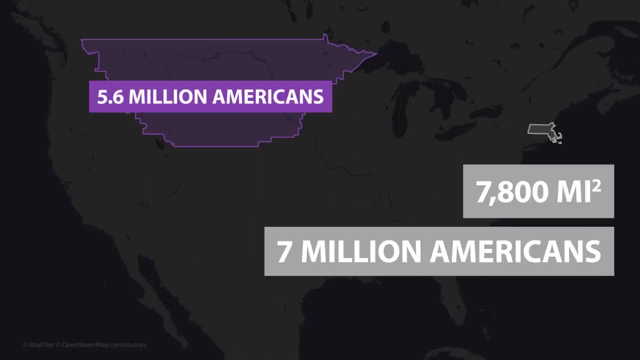 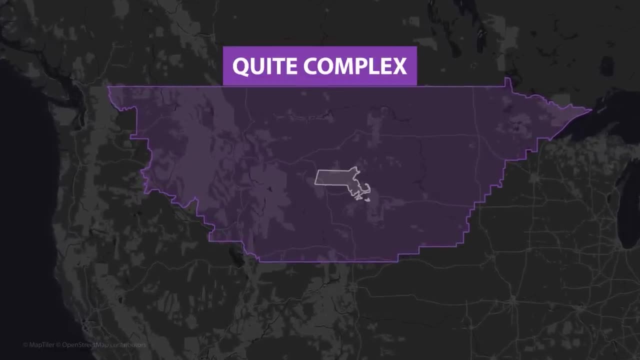 Empty North has 7 million Americans, But of course, while it might seem like the Empty North should have at least as many people as the tiny state of Massachusetts, the entire region is quite complex. The Empty North is really a region of two very different halves In the west. 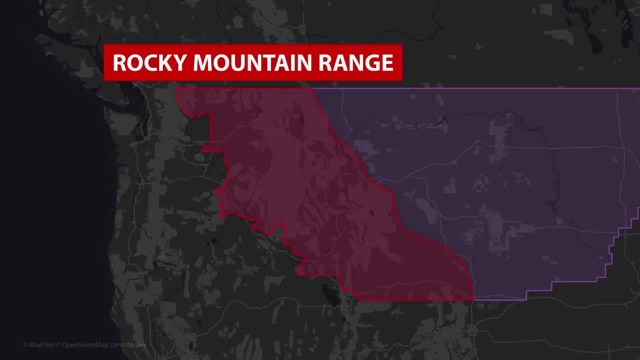 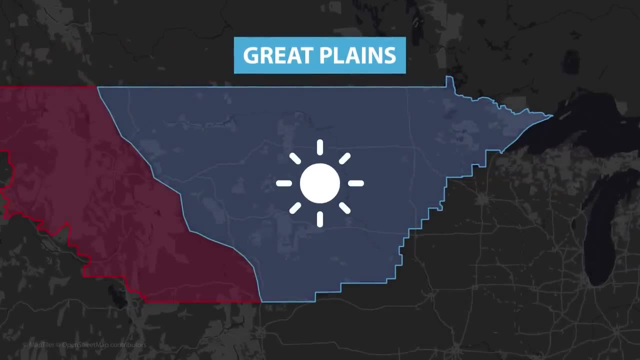 the Rocky Mountain Range creates a complicated area that quite simply is not the easiest place to settle, And in the east, the Great Plains sits within a literal rain shadow of the Rocky Mountains that stretches for hundreds of miles. It's this exact, unique topography that gives Montana its 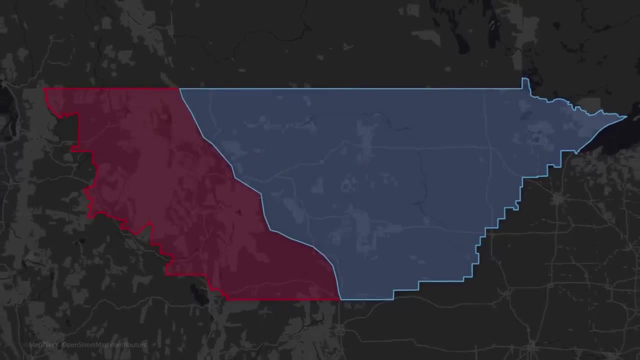 nickname Big Sky Country. Both of these unique geographies combine to create issues in establishing and nurturing large settlements, But, as we'll find out, these are not the only issues can cause. The Empty North is really a region of two very different halves In the west. 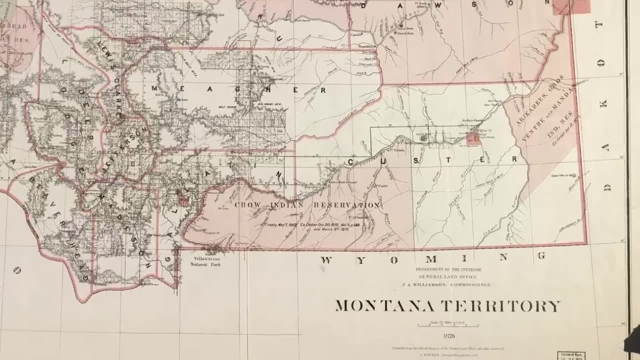 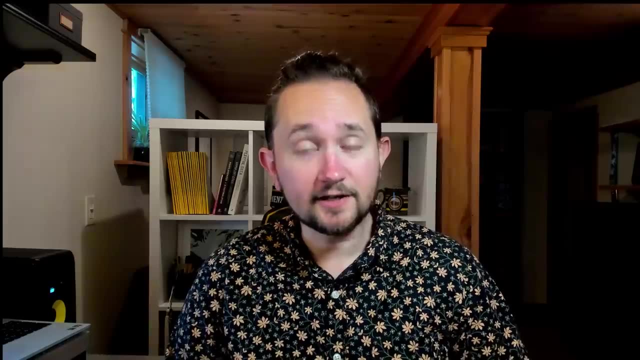 we'll have to dive a bit into the history of the region to find more exact answers. The Empty North is an incredible part of the country, with some of the most awe-inspiring landscapes you can think of, including five national parks. Despite this, however, 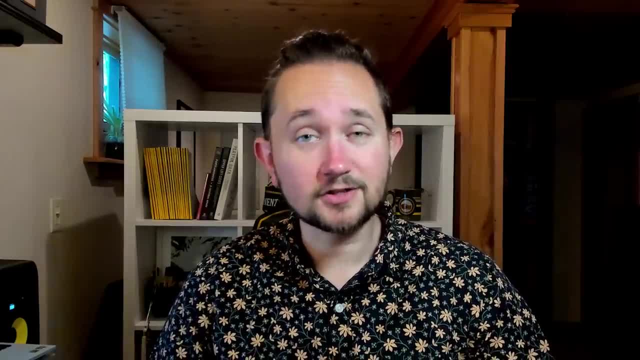 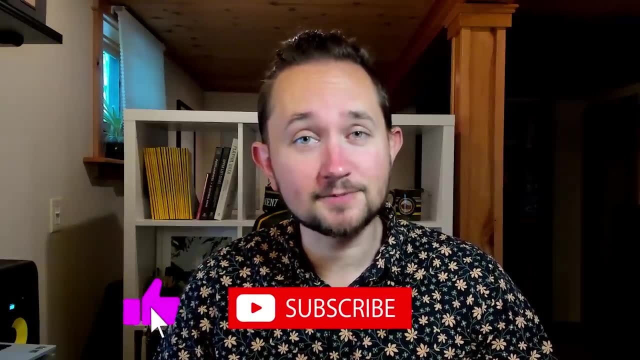 Americans have generally avoided moving to the region at large, And there's a reason for this. But before we get to why there's so few Americans living in the Empty North, if you're enjoying this video, hit that subscribe button. More fun geography videos are just a single click away. 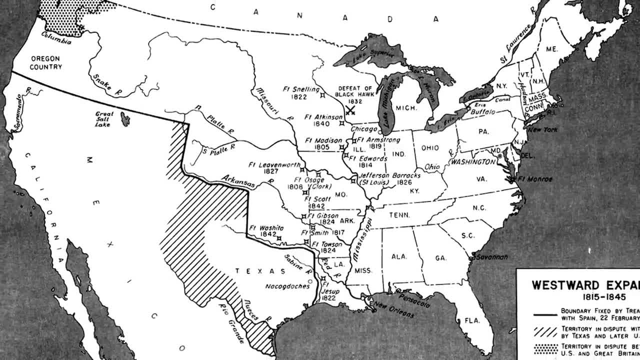 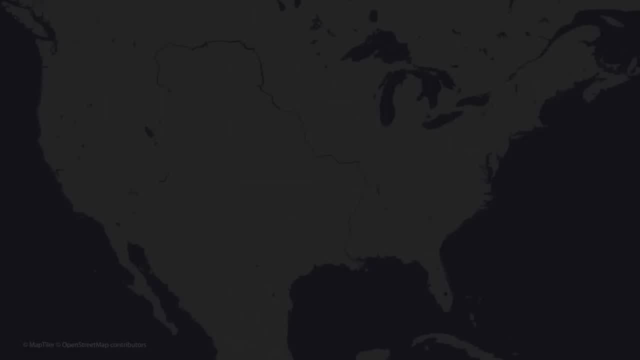 The history of this region specifically can be broken out into three major expansionist events within the United States, And each of these events ended up in the same manner, with the gradual push of Americans from the densely populated eastern shore to the western, more rugged and rural areas. 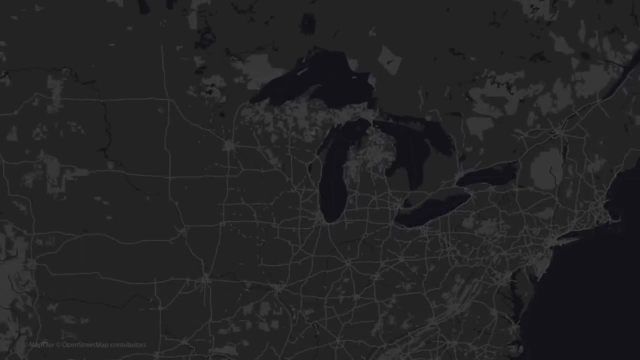 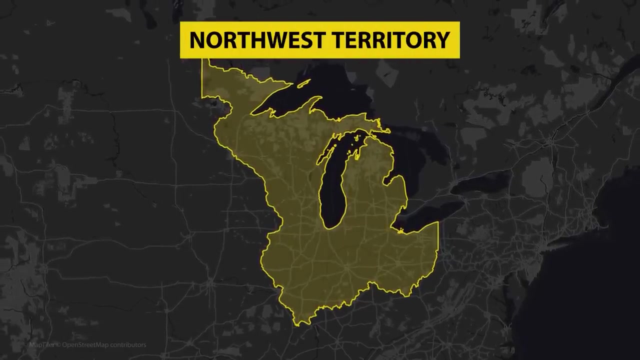 of the country. Shortly after the United States won its war for independence from Great Britain, it found itself with quite a bit of extra land in what was then called the Northwest Territory. This was the land that extended all the way from modern-day Ohio in the east. 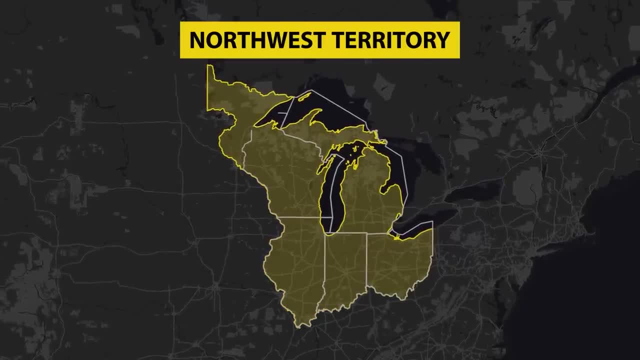 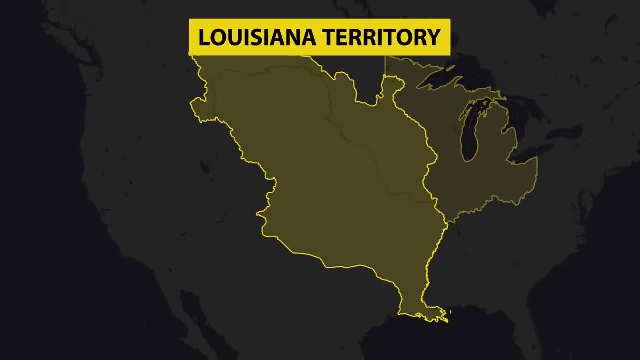 through the Great Lakes region and to the very northern edge of the state that we call Minnesota. today, Happening at about the same time, the United States would purchase the Louisiana Territory from France, effectively doubling the amount of land the US would claim to own. 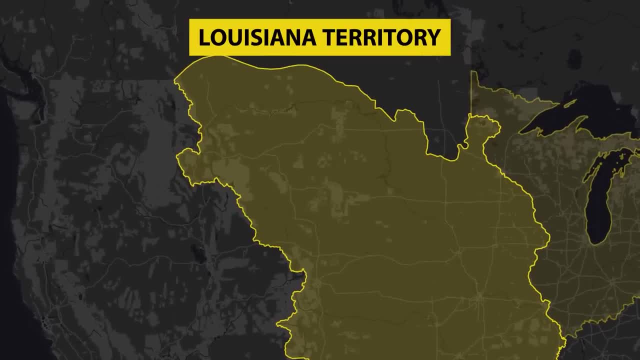 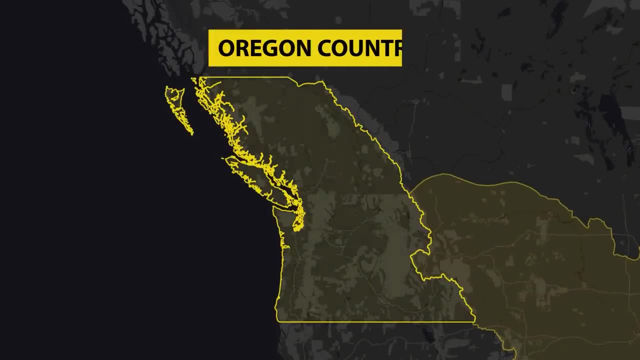 Most of this newly acquired land, of course, would be in the northern region of the current contiguous United States And finally, at the end of it all, the US and Great Britain would compete for what was then called the Oregon Country, which would eventually be split in. 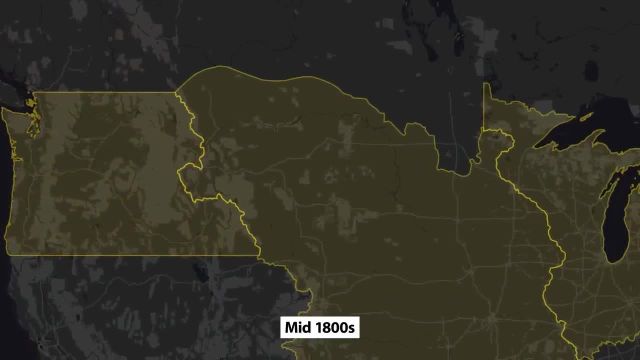 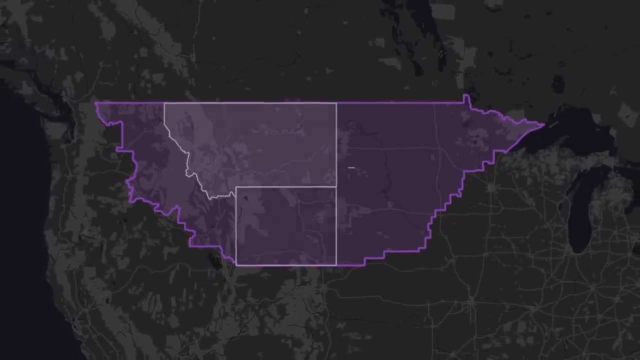 half between the two By the middle of the 1800s, would effectively own the entirety of the empty north. But despite owning this region, the core states of Montana, Wyoming, North Dakota and South Dakota would take quite a long time to. 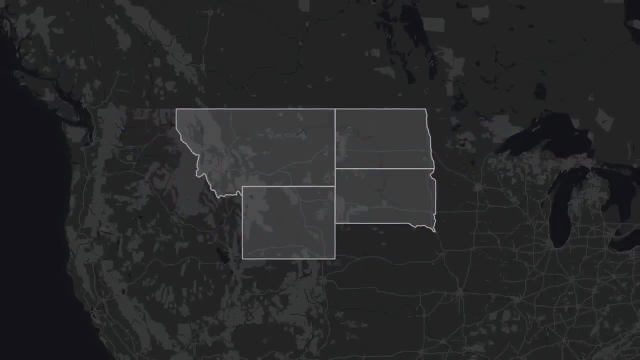 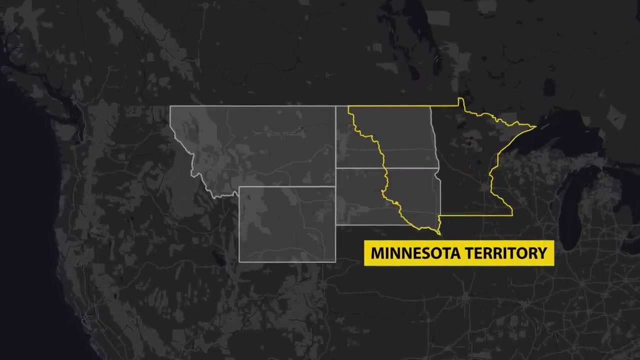 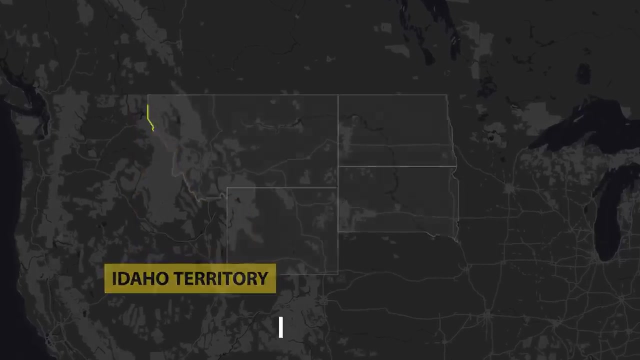 get formally organized. At one point in time, portions of these four states were part of the Northwest Territory, Wisconsin Territory, Iowa Territory, Minnesota Territory, Nebraska Territory, Oregon Territory, Washington Territory and the Idaho Territory. It would take until the late. 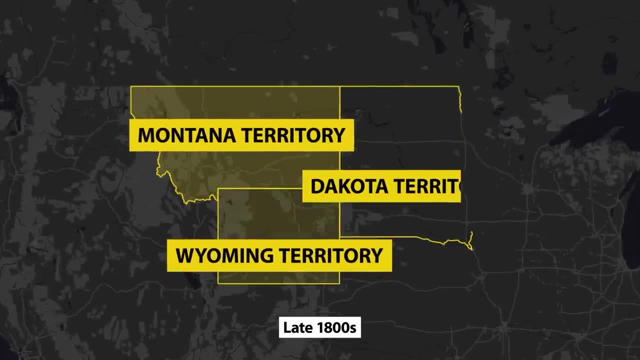 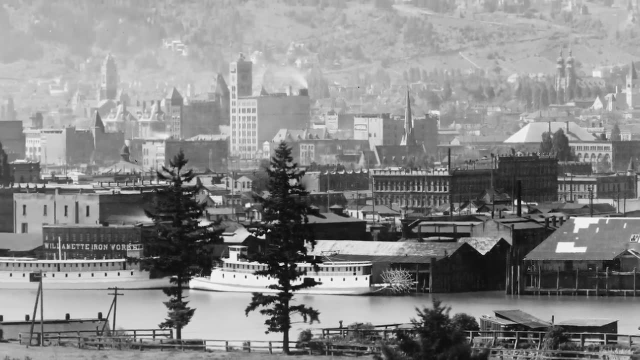 1800s for the Montana Territory, Wyoming Territory and the Idaho Territory to become part of the Wyoming Territory and Dakota Territory to be formally organized. And if there's one thing that we know about these early territories, it's that they were usually propped up by boosters within. 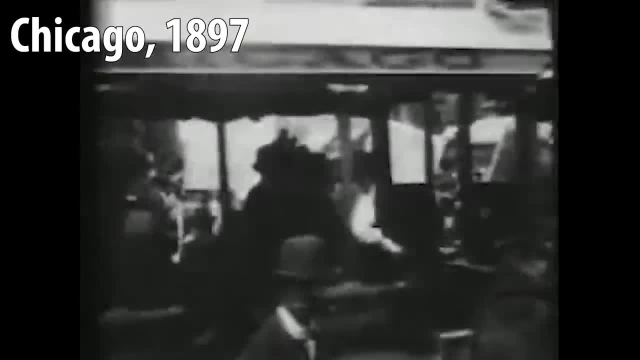 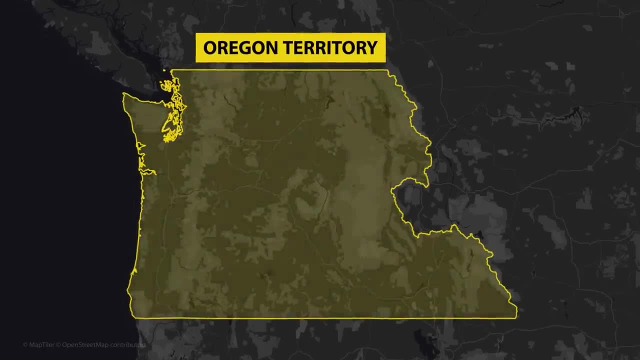 the core settlement of the respective territory. These boosters would strive to get people to move to the general area of the major population center in order to amass an economic center- The Oregon Territory, for example, despite consisting of modern-day states of Oregon. 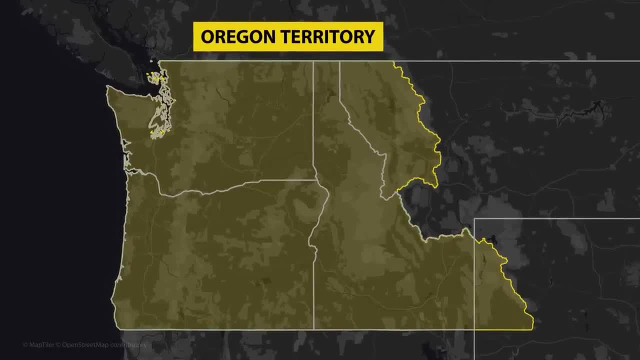 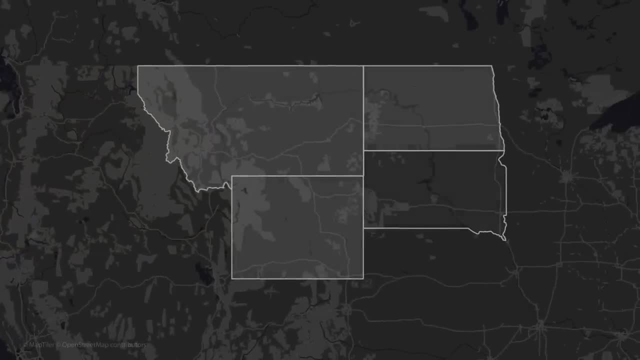 Washington, Idaho and parts of Montana and Wyoming would primarily draw people to the Willamette Valley, the home of modern-day Portland. Oregon, Montana, Wyoming and the North and South Dakota didn't have these early boosters in the same way that many of the other. 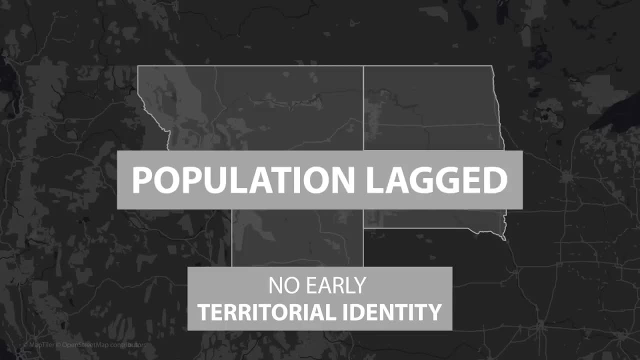 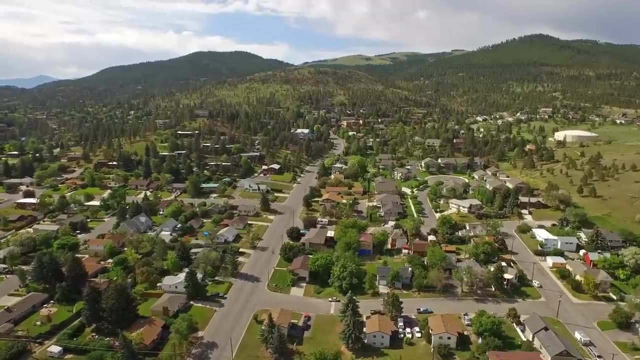 territories did and therefore population lagged during the early push to get Americans to move west. Despite not getting very many people in the early days of the American migration to the west, there's still been plenty of time to get more people to move to the empty north today. 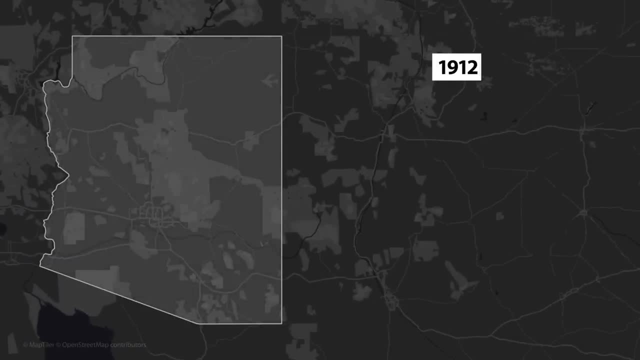 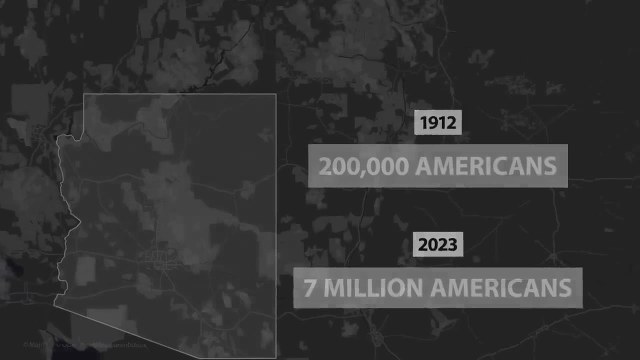 After all, Arizona wouldn't even become a full state until 1912, when it had about 200,000 people living in it. Today, however, Arizona is home to the most populous state in the United States, home to over 7 million Americans, larger than the entire empty north, despite being far. 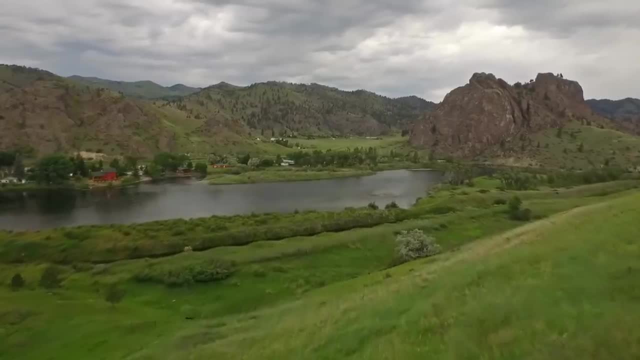 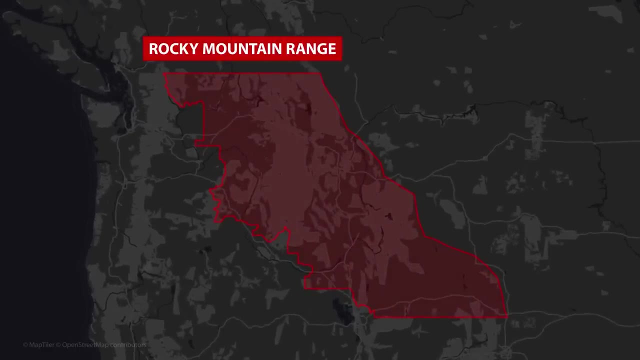 smaller in size, And the reason for this can kind of be boiled down to two major reasons: topography and climate. On the western side of the empty north, the rugged Rocky Mountain range breaks up the relatively few areas that would be habitable. This creates a natural limiting effect. 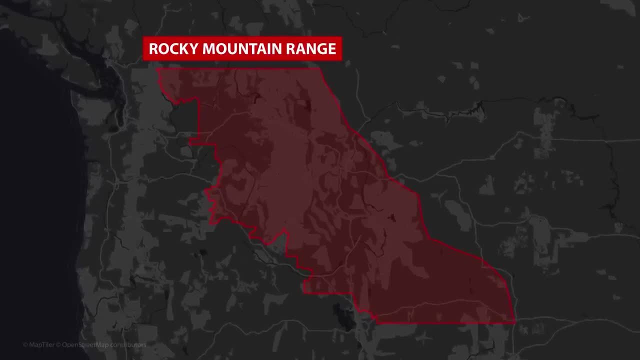 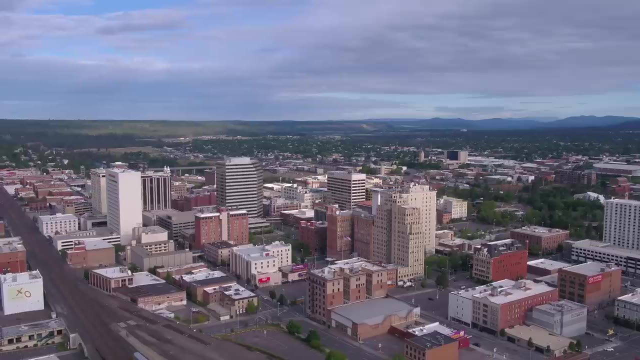 That's not to say that larger cities can't exist in the western portion of the empty north. After all, the Spokane metro region, home to nearly 600,000 people, would comprise the largest city in our region. But Spokane also exists just to the west of the Rocky Mountains, not within them, And this follows. 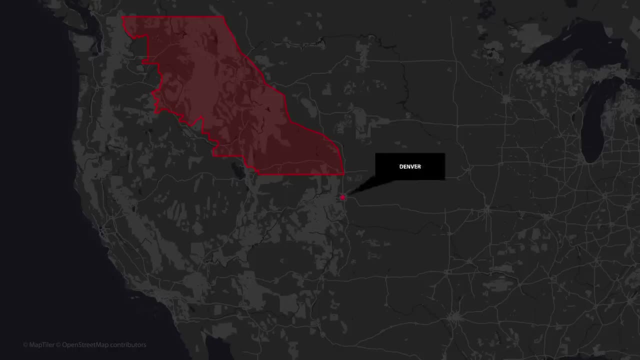 a similar pattern for even cities outside of the empty north. Denver, Colorado Springs, Salt Lake City and Boise are all at the base of either the eastern or western side of the range. Even in Montana, a rugged and rural state if there ever was one, the largest city of Billings is well east. 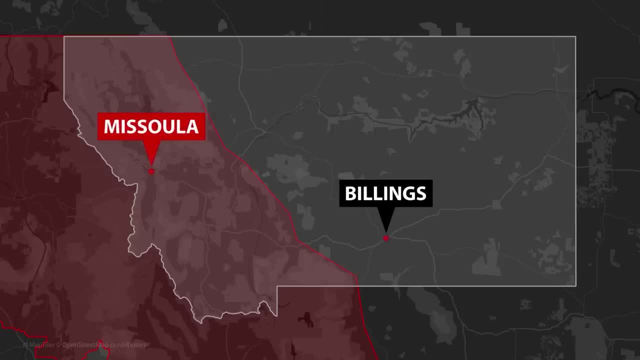 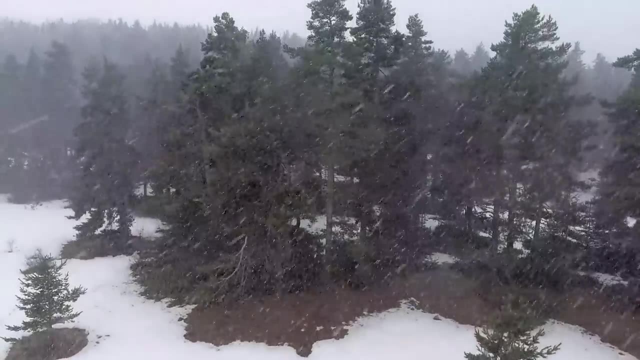 of the Rocky Mountains. Missoula, Montana, is perhaps the largest city. that's entirely within the Rocky Mountain range but is only home to about 117,000 people. And, of course, the other issue at play within this region is quite simply the climate. 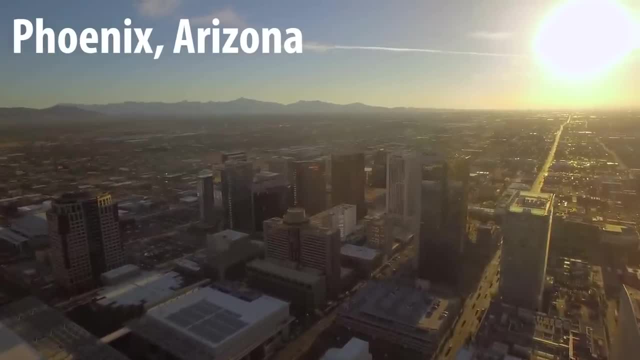 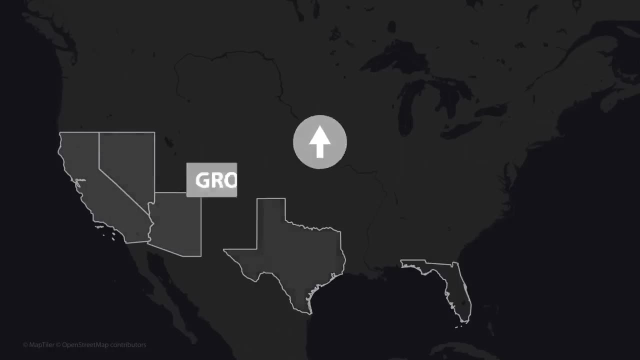 Americans have proven time and time again that they would rather live in warmer, sunnier areas of the country. It's for this reason that places such as California, Arizona, Nevada, Texas and Florida have grown tremendously over the last few decades. The empty north, however, can get quite. 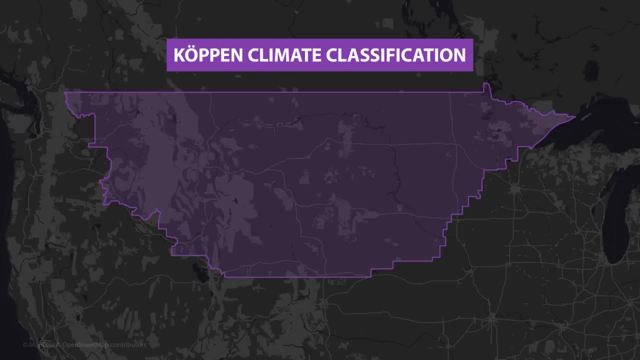 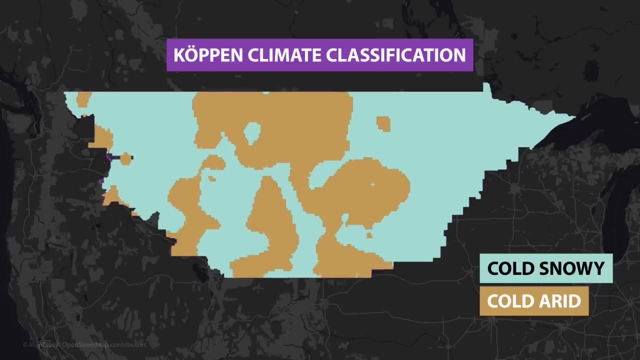 frigid. According to the Koppen method of determining climate across geographies, the entire empty north is a complicated mishmash of cold snowy regions and cold arid regions, and little else in between. The simple reality is that most Americans don't seem to be willing to brave that. 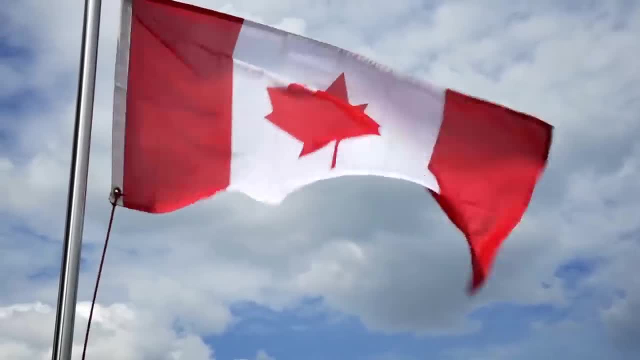 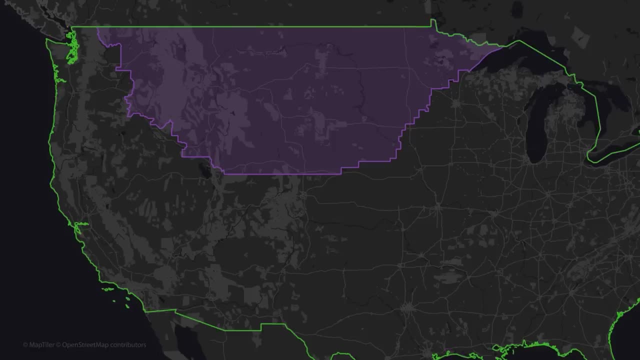 kind of weather, which is interesting because Canadians seem much more tolerant of it. While this video is about the empty north of the United States, it needs to be pointed out that if we look just north of this region into Canada, there exist two major Canadian cities. 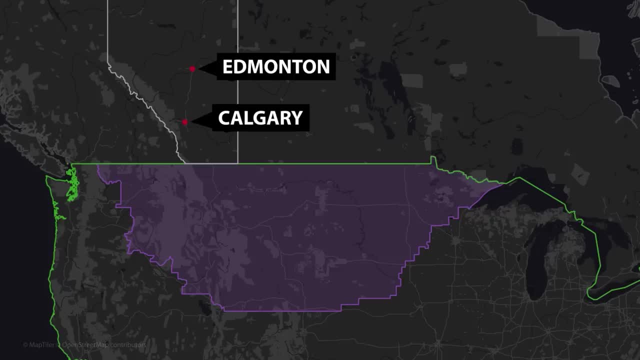 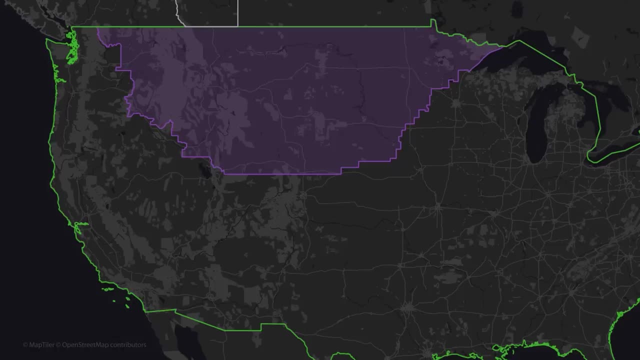 Calgary and Edmonton, And within Canada, those two cities make up the fifth and sixth largest metro regions respectively. If the United States had its fifth and sixth largest metro regions within the empty north, it would have an additional 13.5 million people. 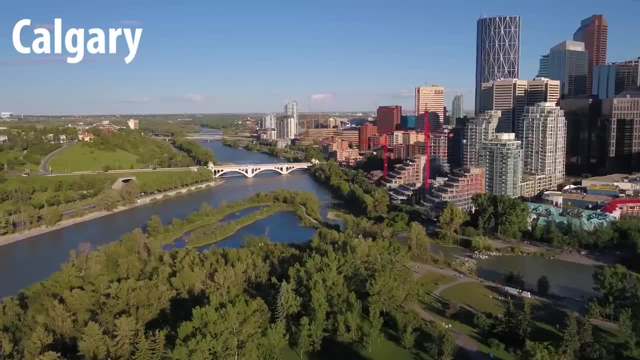 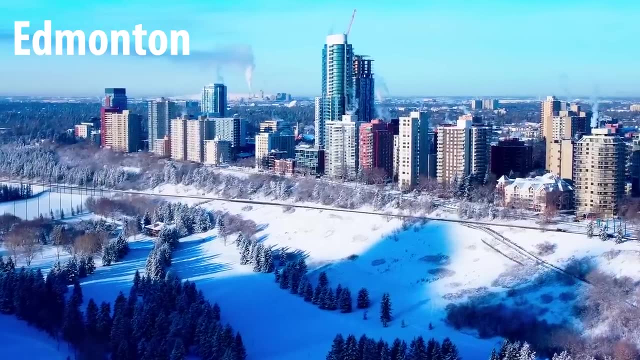 the size of Houston, Texas and Washington DC, And while there's definitely a longer video on why Calgary and Edmonton are so large with respect to their geographic location, it really can be summed up as a byproduct of the Canadian oil industry In the middle of the 1900s large 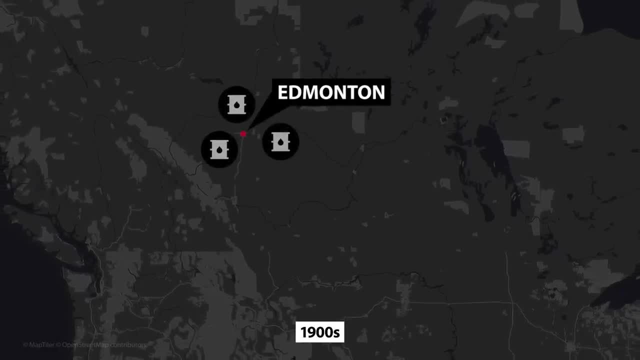 quantities of oil were discovered outside of Edmonton, which brought a large industry to the city And Calgary made for a convenient location for additional oil industry services, as well as an easy location to ship oil to Vancouver, BC and the United States. So if you're looking for, 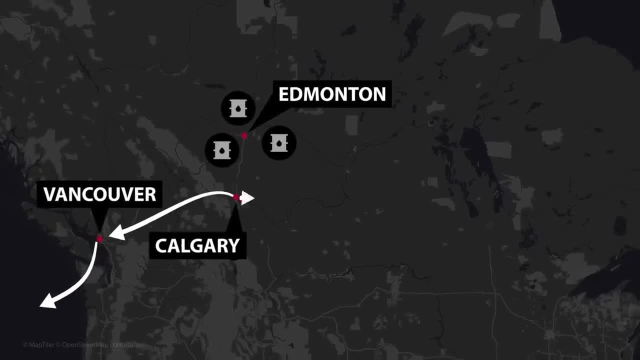 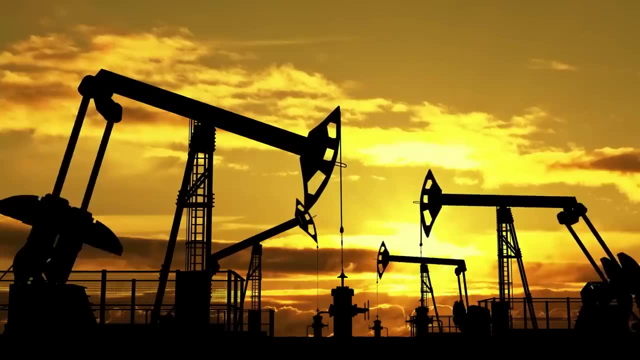 a convenient location for additional oil industry services, as well as an easy location to ship oil to Vancouver, BC and then Asia in the west, to Toronto and Montreal. in the east or south to the United States, The empty north does have oil fields, but ones that aren't nearly as large. 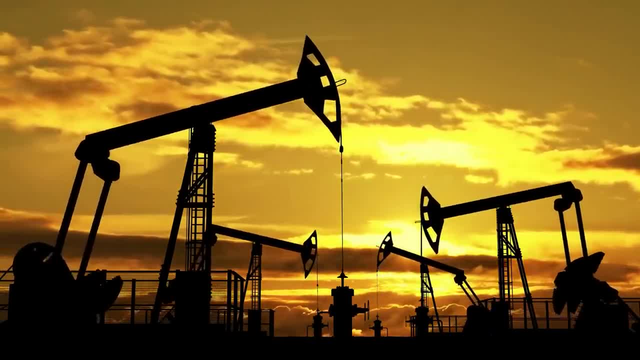 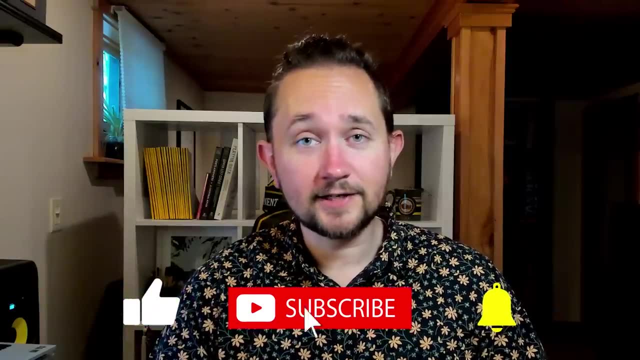 or as easy to extract, and therefore it has not garnered nearly the same population around them. The empty north of the United States could have more people living in it, but a slow start to settlement, lack of industry, cold climate and difficult terrain have all combined to.